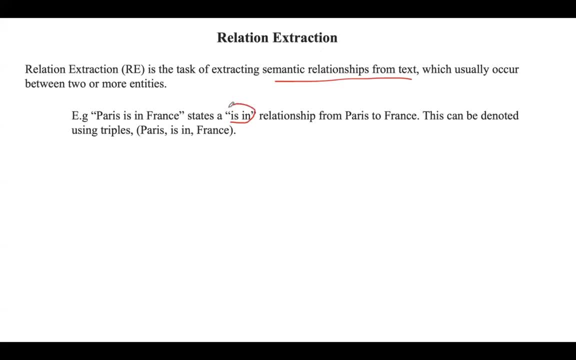 is in France. It states that Azen is a relationship from Paris to France. So here Paris and France are two entities and the relationship between them is Azen. So you can represent this with a triple. So triple means here we will take: 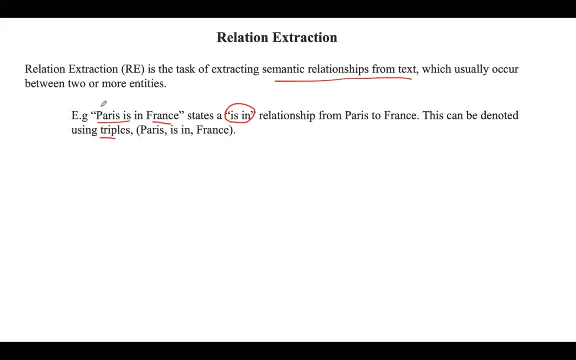 entities, Entities from the sentence and the relationship between them. So entities in the sentence are Paris and France and the relationship is Azen. So we are representing sentence in the form of triple like this. So in our previous video we saw what is meant by information extraction. 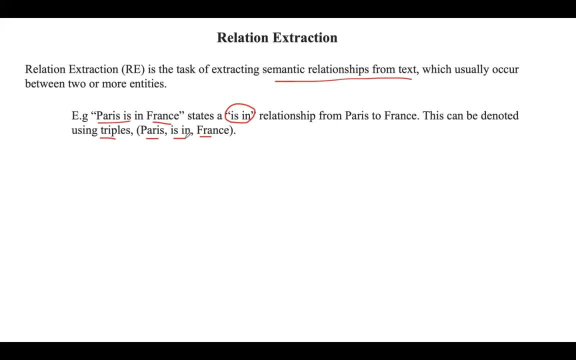 So information extraction is a field of extracting structured information from natural language text, right? So we can use this information In various fields or various NLP tasks like knowledge graphs, question answering system, text summarization, etc. So here we can say that this relation extraction is a subfield of information. 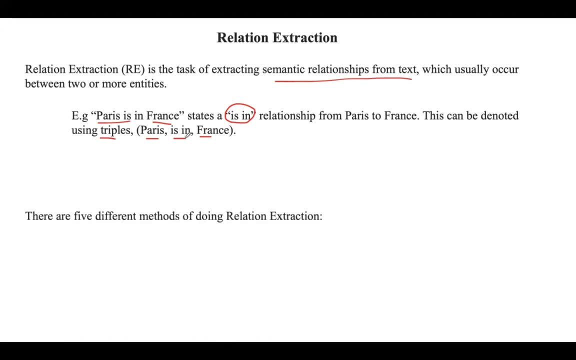 extraction. There are five different methods to perform this relation extraction. The first one is rule-based, Second one is weekly supervised, Then supervised relation extraction, distant supervised relation extraction and unsupervised relation extraction. So we will see them one by one in this lecture. So, coming to the first one, rule-based. So using this approach, 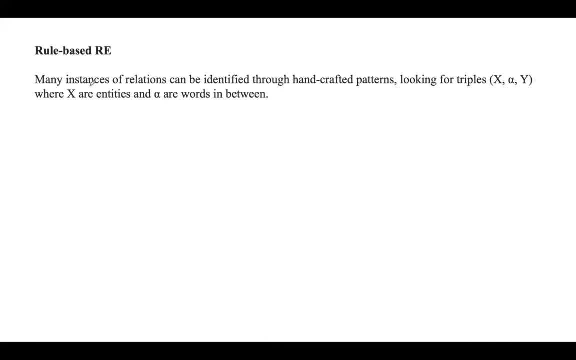 we can identify different relations or many instances of relations with the help of handcrafted rules. So if you represent them by, with the help of this patterns or rules, you can identify different relations. Then they look something in the form of triple like this: X, alpha and. 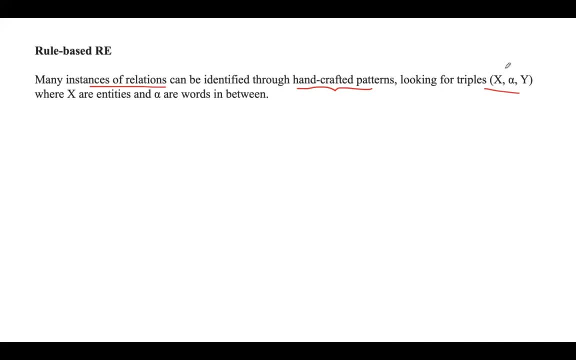 Y. So just now we saw how to represent a triple. So here X is nothing but it is. X and Y are entities and alpha is the relationship between them. So if you take the previous one, So here X is nothing but Paris, Y is nothing but So the sentence is: Paris is in France. So 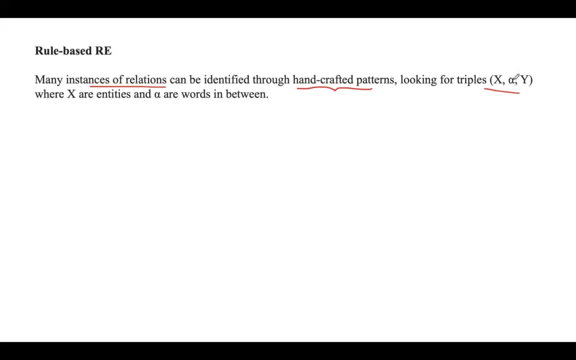 X is Paris, Y is France and alpha represents that is Asian. Only looking at keyword matches will also retrieve many false positives. So there are problems of false positives because the same word, it may have more than one meaning. So in order to resolve this, we can filter the entities on using either name: named entity. 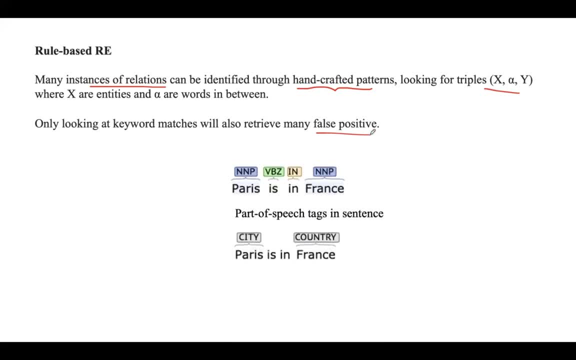 recognition. That means only So if you take this second one. So here we need to retrieve: only city is in country, instead of taking it as Paris is in France. So we are assigning the entities to every word in the text and based on that will retrieve, or else you can. 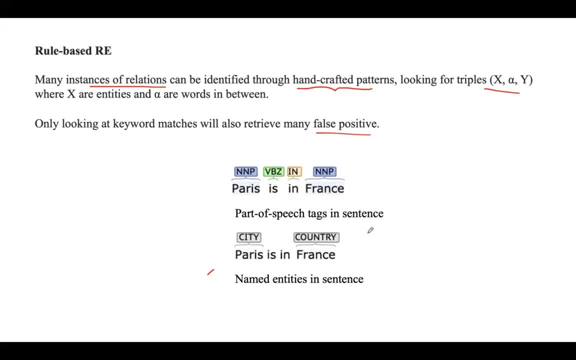 use POS tags in order to remove additional false positives. So by assigning POS tags also, we can identify what that word refers to, whether it is a name of, whether it refers to verb or whether. So if you take this second one, So if you take this second one, So if you take this, 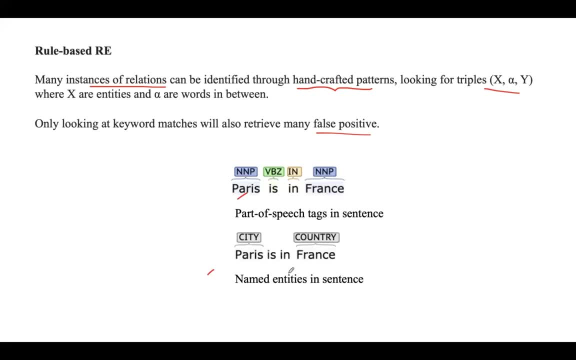 third one. So if you take this third one, So if you take this third one, So if you look at, the answer is whether the word is now similarly here. if you take Washington, Washington can be name of a person or it can be a location. So in order to identify the 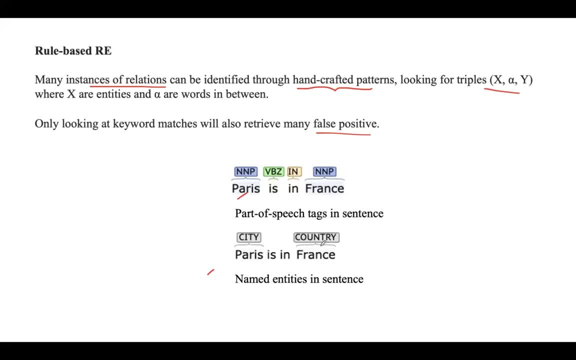 differences, it's better to go with these two kinds of approaches. So these are some examples of doing word sequence patterns, because the rules specifies pattern following the order of the text. but unfortunately these type of rules they fall apart for long range patterns and sequences with great variety. so these type of things they comes under word. 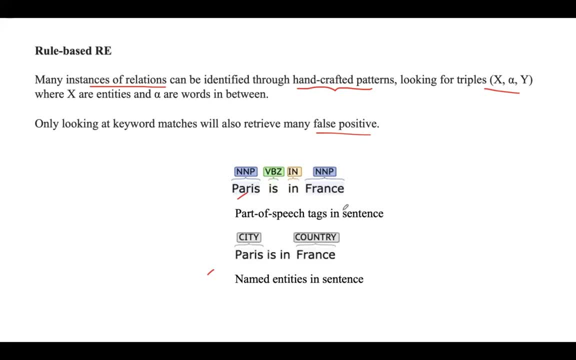 sequence patterns because why they are following the order of text. so based on that, only based on the order of text, we are going to define the pattern. but sometimes this method it may not work, especially if the pattern or if the sequence is very long. so if you take this, 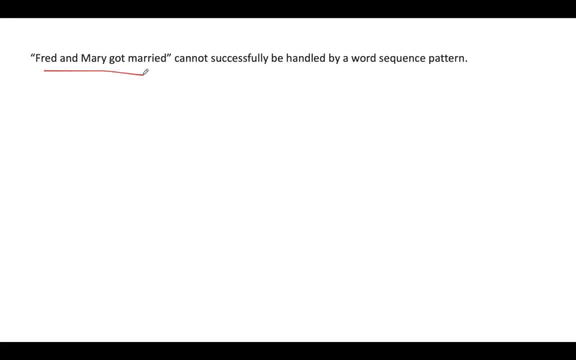 sentence fred and mary got married, so it cannot be handled by the word sequence pattern. so for that. so instead of using this named- ntr sorry named- entity recognition or part of speech tagging, you can go with dependency parsing for these type of sentences. so here: fred and mary got married. 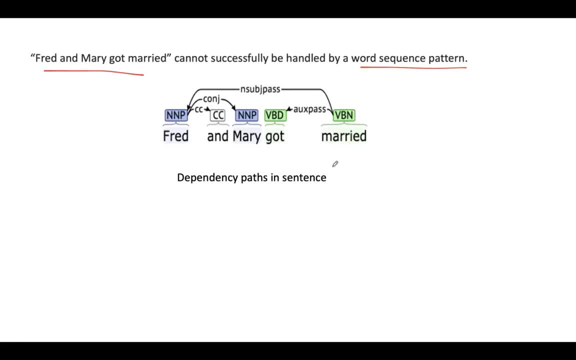 so this is the sentence. so for this, you you need to find out dependencies or relationship between the words in the sentence. so instead of so, we can make use of dependency paths in the sentence, knowing which word is having a grammatical dependency on other words. so this: 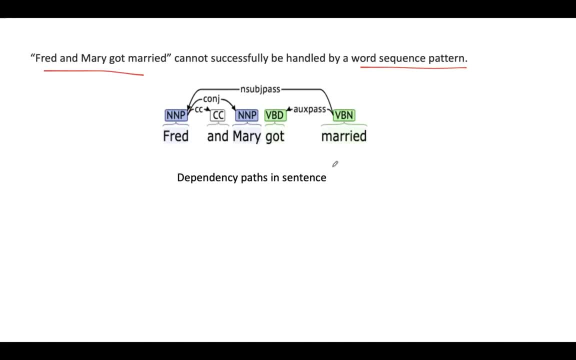 can greatly increase the coverage of the rule without any explanation. so yeah, we have seen earlier two sentences right, and there was a commercial more effort. so here you can see there's a relationship in even transform the sentences before applying the rule. so if you take a sentence as the cake was baked by harry or the cake which harry baked, so instead of writing this you can just simplify the sentence into harry baked the cake. so this became quite simple, right compared to previous two sentences. so we can even transform the sentences into: above the did we such a cake? 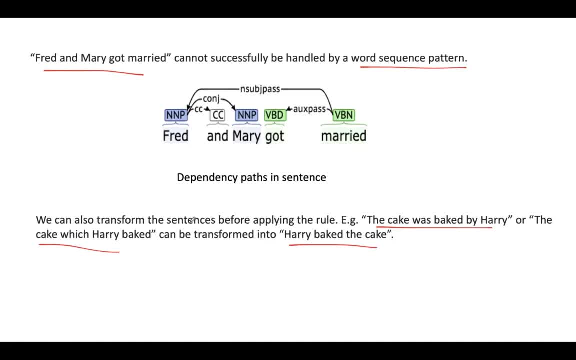 became quite simple, right compared to previous two sentences. so in that way you can even transform the sentences before applying any kind of rules and after transformation again, here we are changing the order to work with our linear rule, so we are removing redundant modifying words in between. so here you. we are removing words like was or by. here it is which. 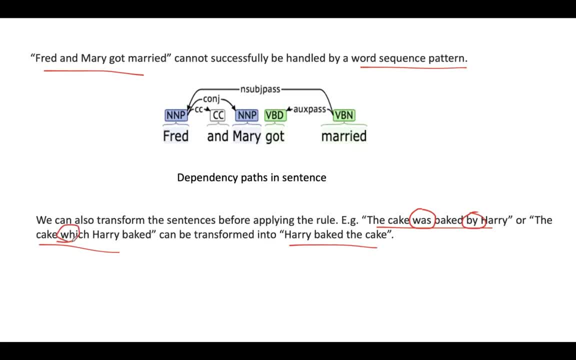 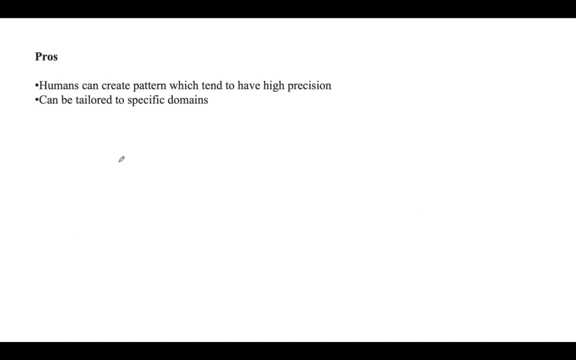 okay, in this way we are changing the order, coming to the advantages, human can create patterns which tend to have high precision. so here the patterns or the rules. so here the patterns or the rules. so here the patterns or the rules. they are created by humans, so because of that, it can have, or they can produce high precision. 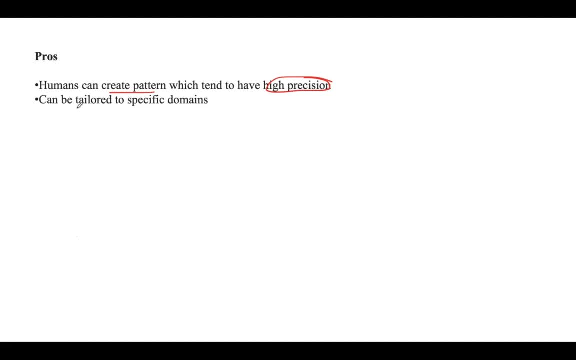 and it can be applied to specific domains. so even now, so if it can be applied to any kind of domain, a special domain, so if you take computer science, so the for that particular domain we can apply it. if it is medicine that can, for that domain it can be applied. like that, this approach can be applied. 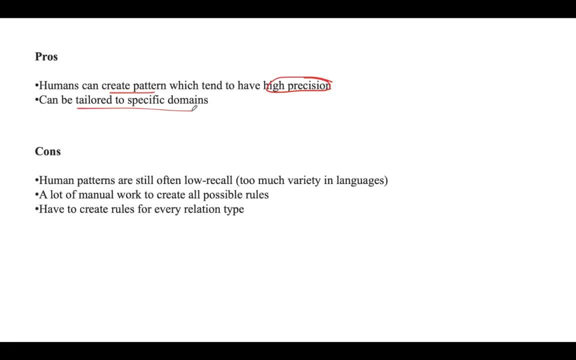 for specific domains. any human to disadvantage is human patterns. they are still often low recall. so because of the variety in languages, so that can be any language. so here, because of that, the patterns which are generated by the humans, they'll produce low recall. so here, advantages: they are producing high precision, but the job is Low recallound soおすすめ. 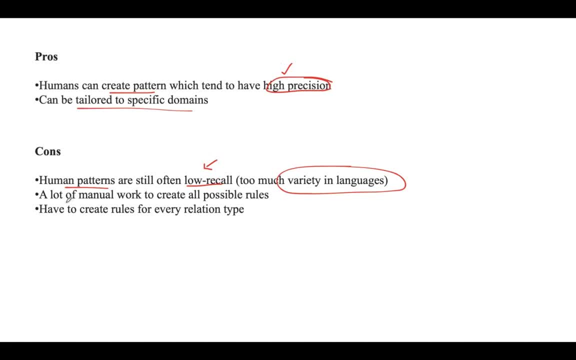 call and as if the things should be done by human, then obviously there should be more manual log, there will be more manual work. so here a lot of manual work is required in order to create all possible rules. and also we need to create rules for every relation type, so based on the type of 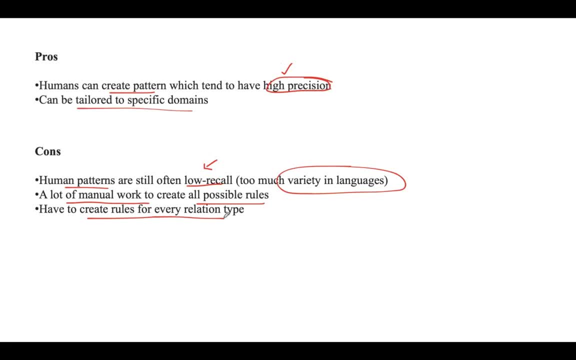 relationship between the words. we need to create rules, so all possible rules should be created. so these are some problems. this one is weekly supervised relation extraction. so here the main idea is to start with a set of handcrafted rules and, based on the rules, we need to find out. 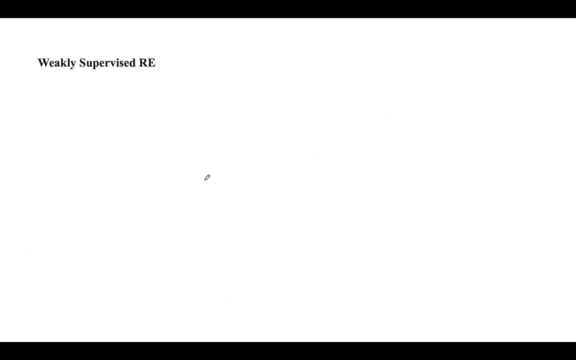 new ones from the unlabeled text data. so this is a an iterative process. we'll repeat the process until we reach end of the text. so, alternatively, you can even start with a set of seed tuples. so we can start with a set of seed tuples and we can start with a set of seed tuples. 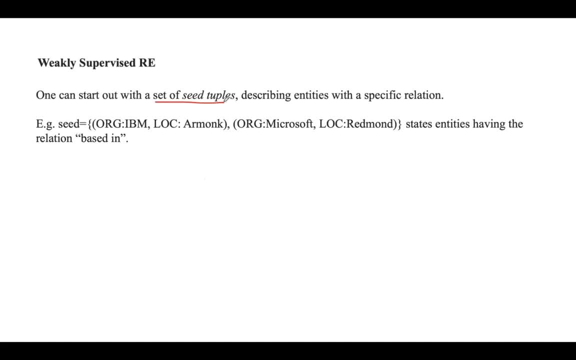 so we'll start with seed tuples and we need to describe entities with a specific relation, so how a seed tuple looks like. so this is the example. so if there, if the sentence is, ibm was located in among or microsoft was located in redmond, then you need to represent them. 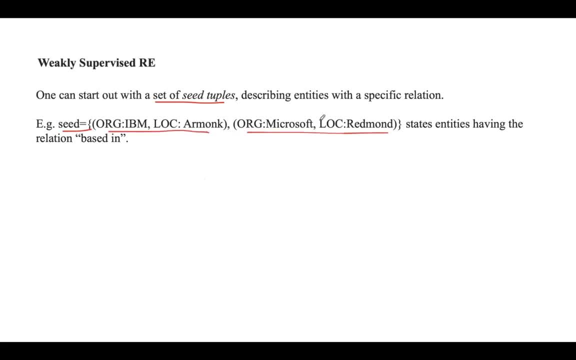 with the help of seed tuple. so this is a representation. so we are describing the entities with a specific relation and the relation between adopted resources based in. so later see the process. so snowball is all example of an algorithm and the process for this is the first. 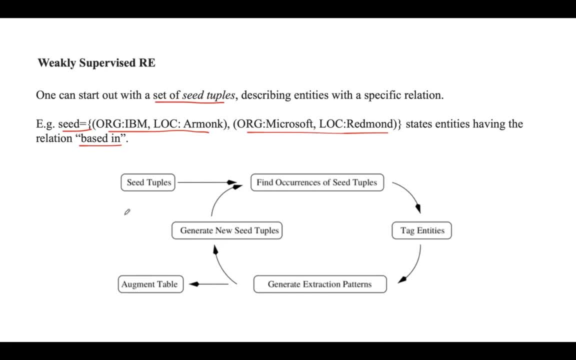 we need to start with a set of seed tuples. ok, so now second step is: so we will take the seed tuple like this and will start with that. next you need to extract occurrences from the unlabeled text that matches the tuples. so take the text. so this is the unlabeled text. now you need to find out occurrences. 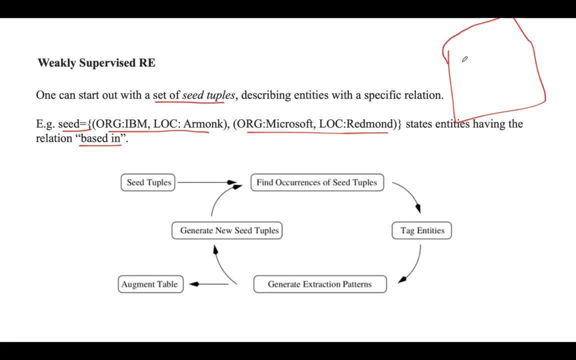 that match the tuples. so find out. say suppose IBM, IBM are mock, so these are the words which are present in the unlabeled text. So these words IBM, Armonk, Microsoft, Redmond, So they assume that they are existing in this unlabeled text multiple times. So in 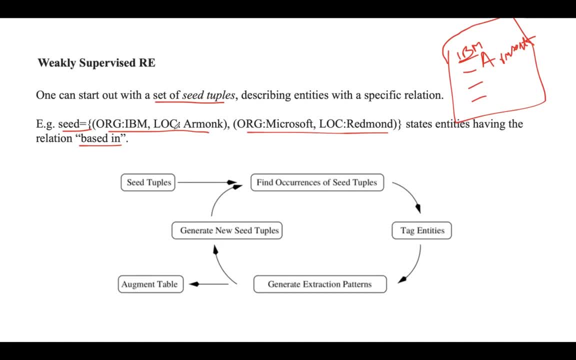 that case you need to match these C-triples, or you need to match occurrences from the unlabeled extract, occurrences from the unlabeled text. So you need to find out whether these terms, they are existing in the unlabeled text or not. If they are found, then you need. 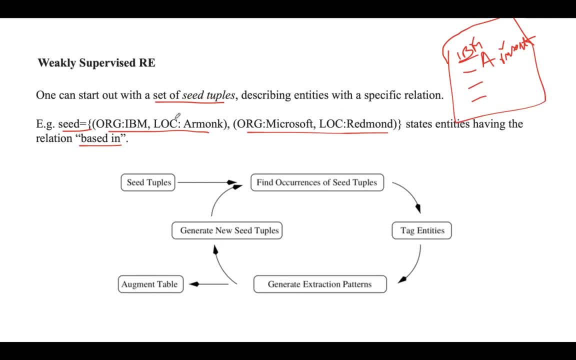 to match them with the C-triples. So if there is a match, then in that case you can extract those occurrences and tag them with named entities. So what we are doing: first we need to check whether the occurrences are existing in the unlabeled text or not. So 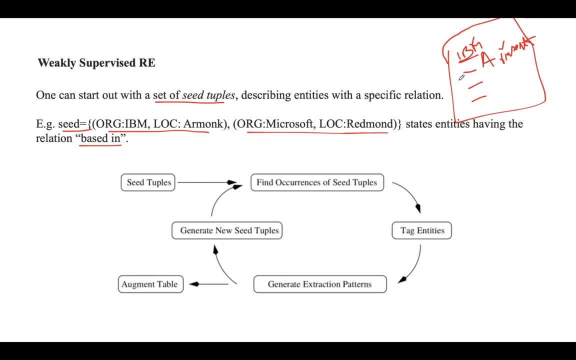 if there are occurrences or the words which are present in this unlabeled text, they match with the C-triples or not entities in the C-triples. So here, IBM, Armonk, Microsoft, Redmond, I assume that they are existing in this unlabeled text. So now, as there is a 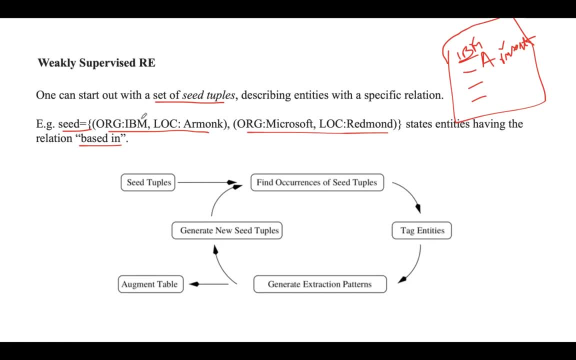 match with the entities present in the C-text. So here you need to extract them and tag them with NER. So extract IBM, So tag them with NER. So extract IBM, So tag them with NER. Obviously, NER will be organization. Extract Armonk and tag them with NER, So as 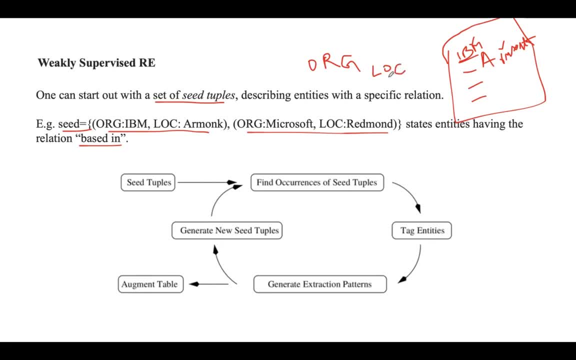 that is a location. NER will be location for that. So, like that, we will extract occurrences or find occurrences of C-triples, Next create patterns for these occurrences. Now we need to generate pattern. So we extracted these words right, So we need to create patterns. 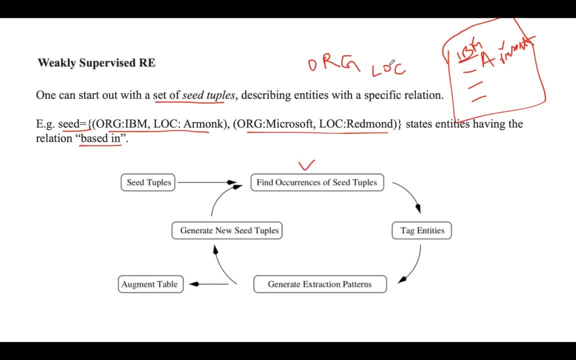 create patterns. So already we have assigned organization entities for these words which are existing in the text. So now, as we have organization and location- So we assigned organization and location as entities to the words present in the text- Now we need to. 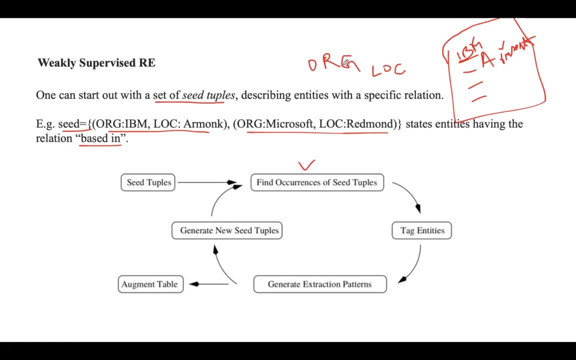 create patterns for these occurrences. So we can create pattern, as organization is based in, Organization is based in location. So that is the pattern which we created for these occurrences, right Then, so named, after finding the occurrences of C-triples. after finding 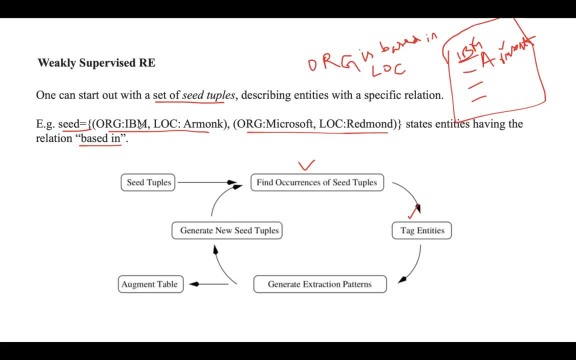 the words or entities which are similar to the entities present in the C-triple, then we need to assign tags entities. So we need to assign tags entities. So we already assigned entities. as for IBM, it is organization among, it is location After. 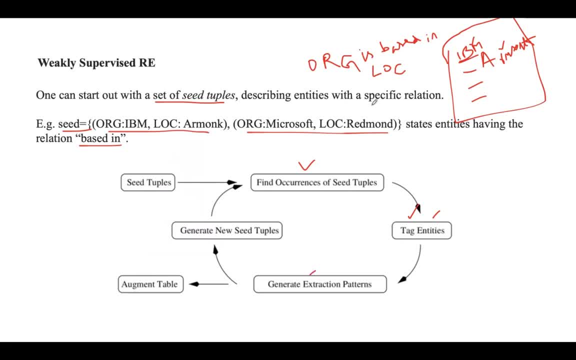 assigning the entities. you need to generate extraction patterns. So we generated new tuple or we created patterns for these occurrences, as organization is based in location. Now next step is generate new tuples from the text. So now find out whether there are any. 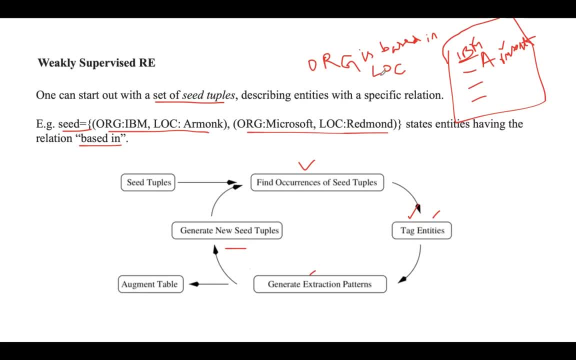 new tuples. If there are two, then we will spend two and three times for each tuple. That is, we can use the one tuple which match with the location and organization, So which match with the pattern which we extracted before. Let's say, we have words like Intel and 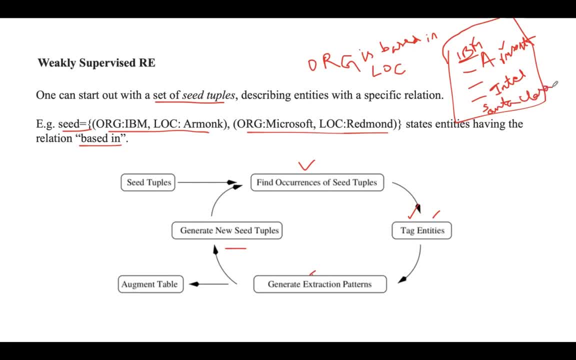 Santa Clara. New words: Intel and Santa Clara. So if, If generate new C tuple, So you can generate a tuple like this by taking Intel, So organization becomes Intel and location will be Santa Clara. Okay, So this is how you can have any set of. 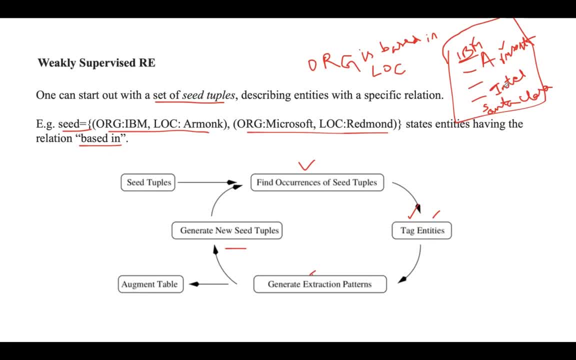 organizations and locations in this new text. So you need to extract everything. So first we extracted this one- Intel, Santa Clara- and as we generated new C tuple like this, So now new C tuple will be: organization is Intel, Location is Santa Clara. Earlier we have 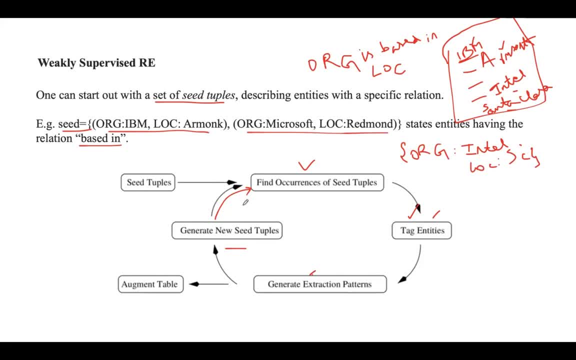 this one. Now we have new one, So you need to add this new to the seed set and so, along with these two, now this also becomes part of the seed set. So you need to repeat this process until you reach end of this text. Okay, Then so, or else say you already reached end of. 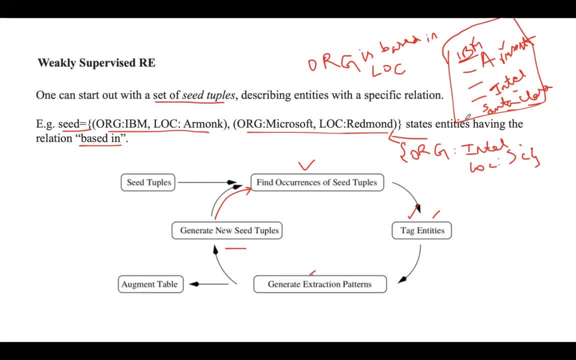 the sentence and end of the text and there are no more entities in the text, Then you can stop the process then and generate augmentation table where will represent all these C tuples which we generated in the process. So this is a procedure for weekly supervised relation. 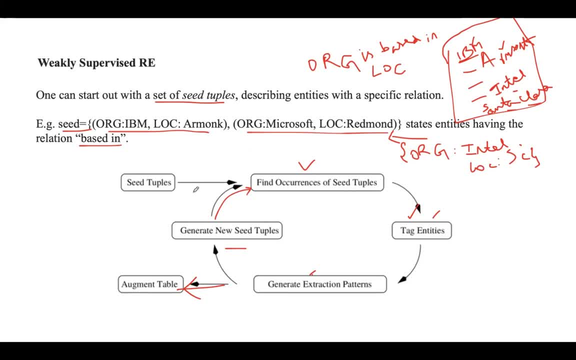 extraction. So coming to the advantages of weekly supervised: here, more relations can be discovered when compared to rule based relation extraction, and also less human effort is required. So, as we are doing everything with the help of the algorithm, less human effort is enough for this.